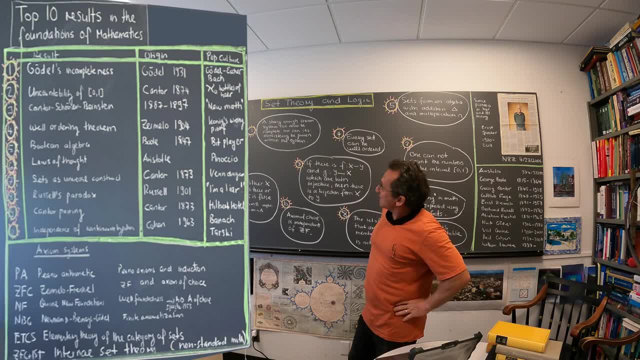 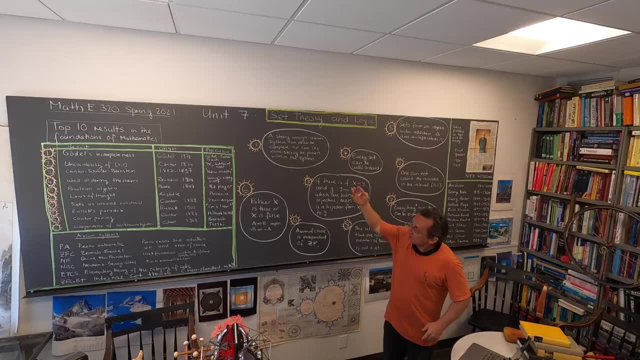 signature here. So for the preparation of this lecture I tried to make a list of the top 10 results in logic or set theory. Definitely the most important one is Gödel's incompleteness theorem. It's very accessible. Also, I have put it on the top because I was also already. 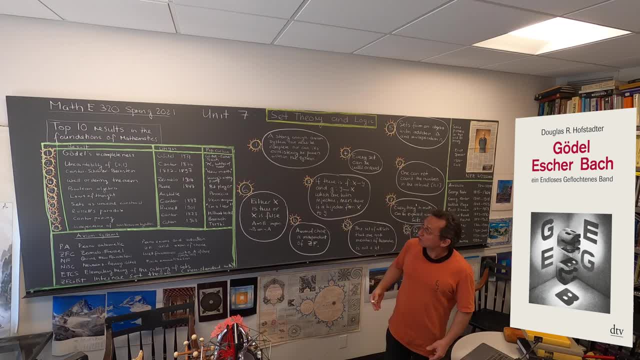 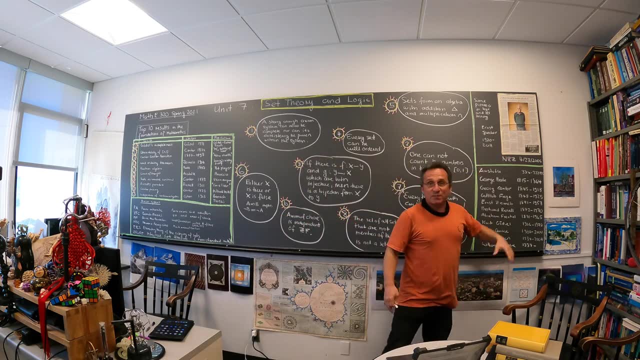 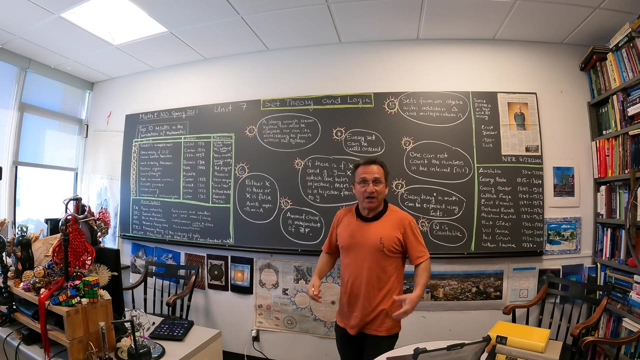 as a high school student. I could read about it, like in Gödel Escher Bach from Hofstadter's book, And it was everywhere. It was in the newspapers, like this Swedish newspaper, and NZZ has often had articles about this. This theorem shatters the dream of Hilbert of building. 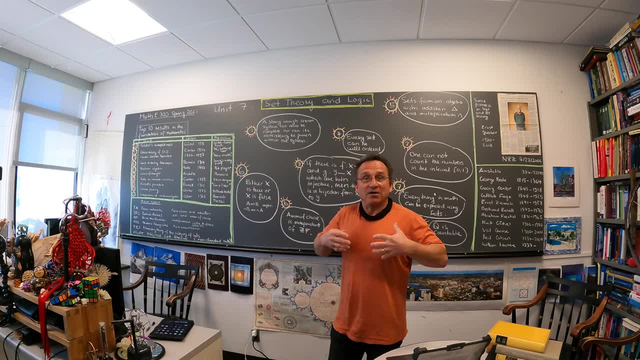 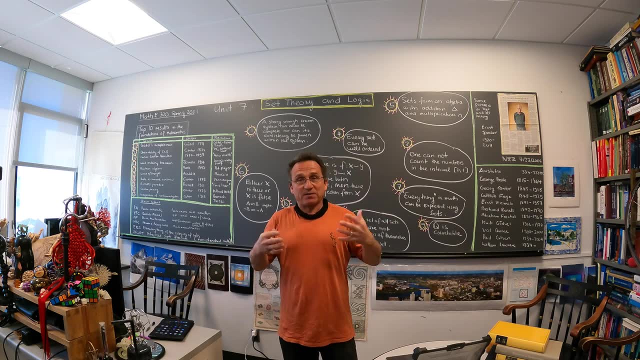 a foundation of mathematics which covers everything. So there's always, if you have a strong enough system, like the Peano axiom system, which we usually take for granted, then there are always results which we cannot really prove. So either we can take its truth. 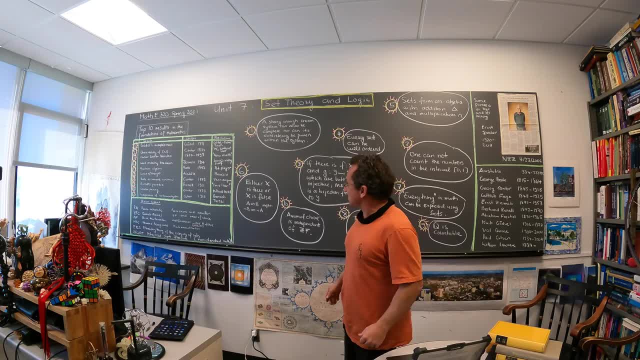 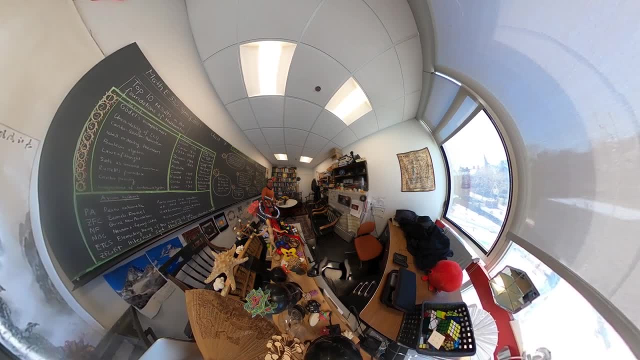 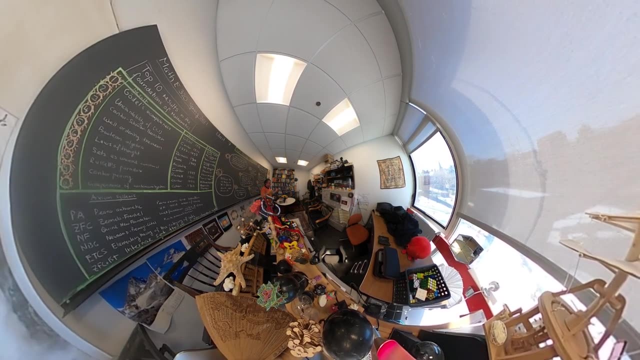 as true or false and both are consistent with the original theory And one of the kind of I put the tenth part, axiom of choice is one of these results which is independent. but also with the axiom of choice or without axiom of choice, you have again a choice to. 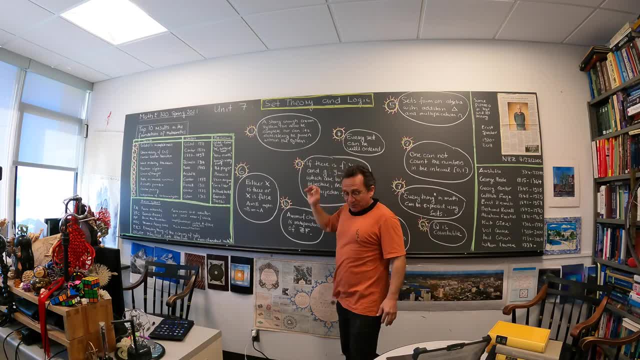 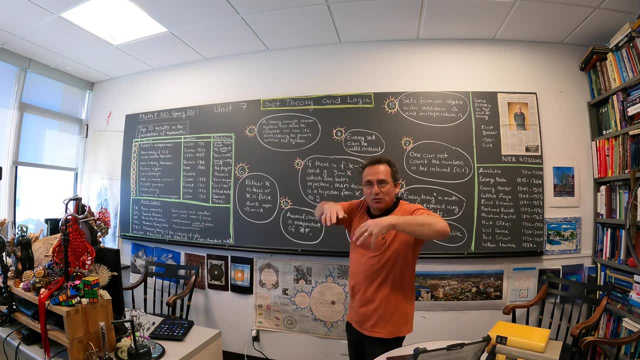 extend mathematics. So it's extremely exciting also that we cannot, in a system which is strong enough, we can prove the consistency of the system within that system. So we have to go out of this system. So we never know, for example, whether our foundational system 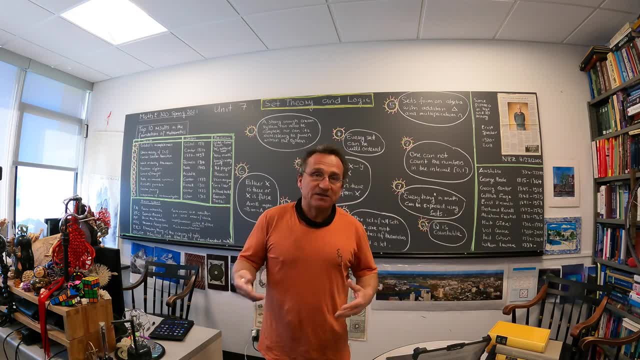 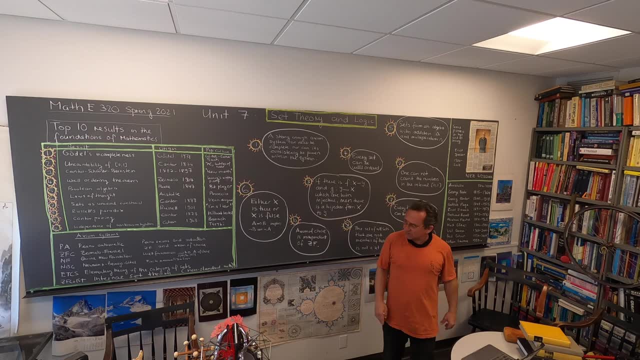 which we usually take for granted, the Semino-Frenkel axiom system. whether this is consistent, It could die tomorrow. There are many alternatives and we have a very, very rich mathematical structure, also in the foundation, so there are lots of alternatives. Mathematicians are. 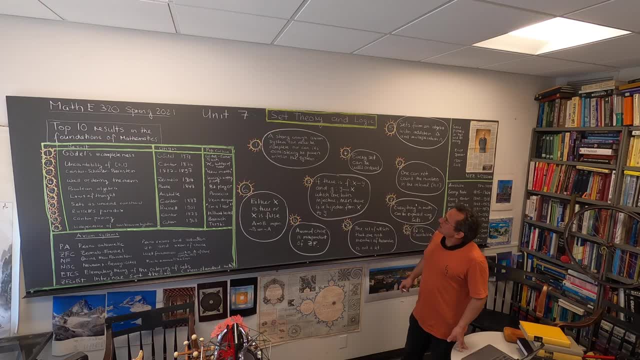 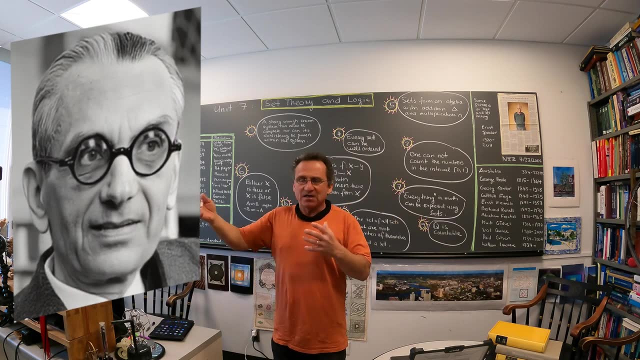 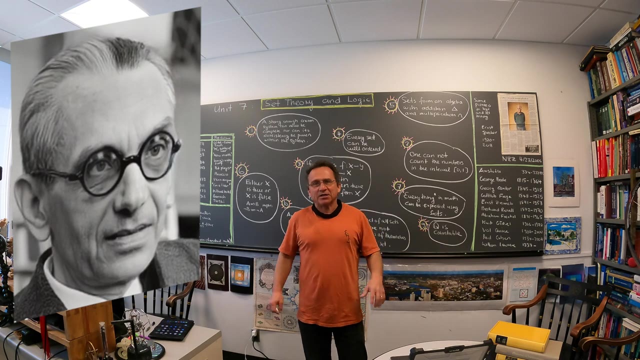 still working on this. So that's number one, a very exciting result. Also, Gödel is one of these figures you know because of his connection with Einstein, Einstein who really was, you know, an icon And Specker who gave this logic what he. 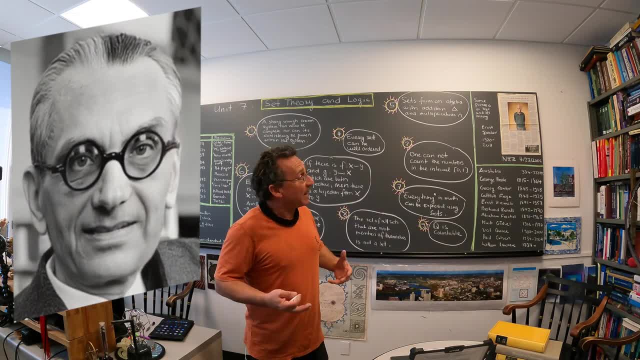 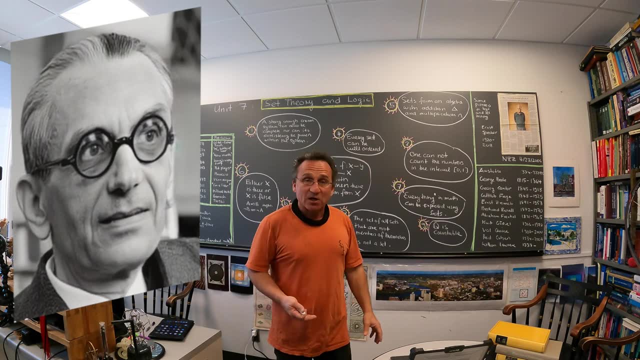 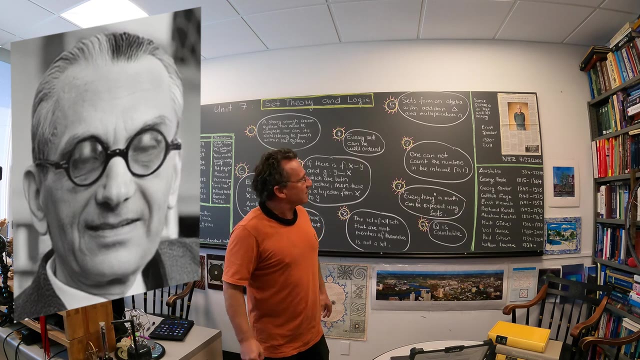 said once that other mathematicians, like Paul Berner, who he knew, was actually thinking that this is true. He was thinking even because probably quite a few mathematicians thought this is the case but also thought that this is not provable. that's so difficult And 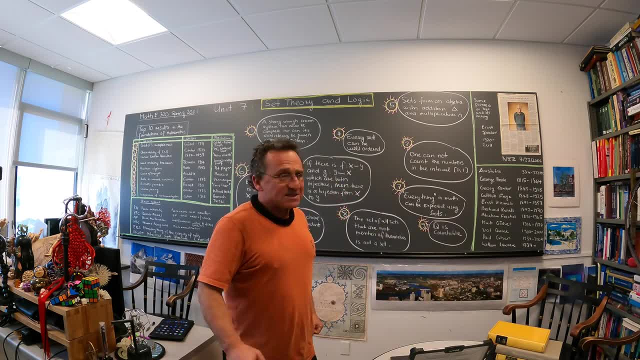 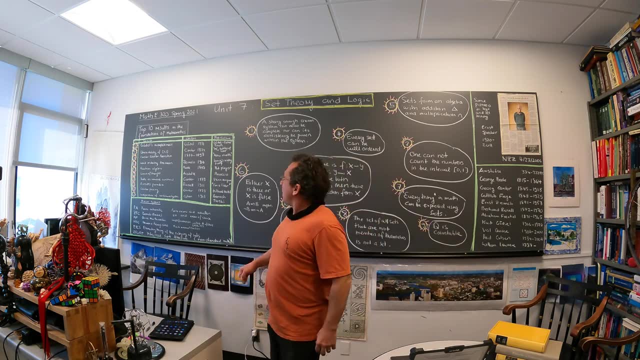 Gödel really succeeded with proving this. It's a very interesting story. also, you know that at that time, when Gödel announced that result in 1931, then others like Zermelo were very, very upset, And so Zermelo even gave a talk just after Gödel at that conference. 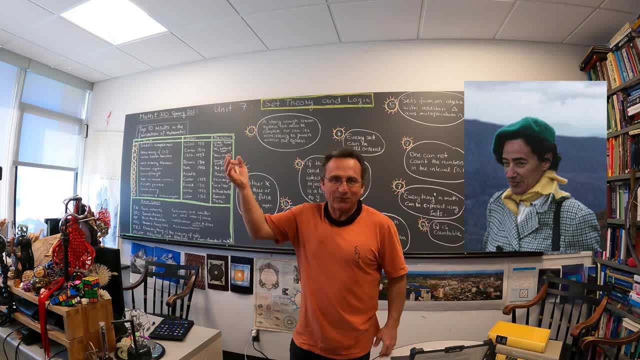 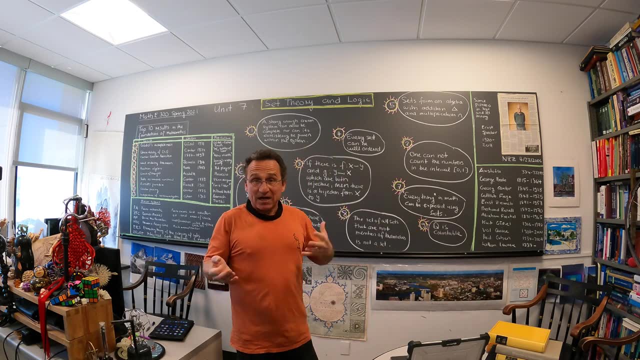 So this story has been told by Olga Tautsky-Toth, who I know from Caltech. And then the next thing is also very exciting. It's something you can, Yeah, Also understand very early on that there are different infinities, So there are infinities. 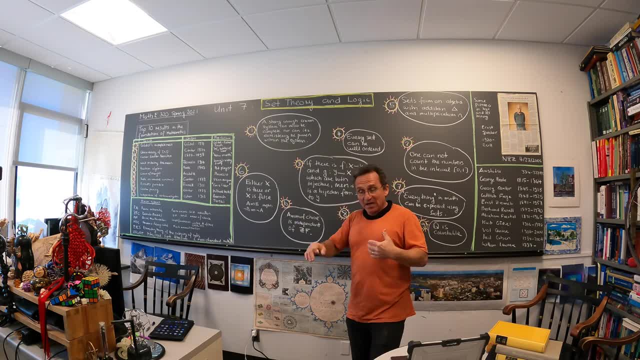 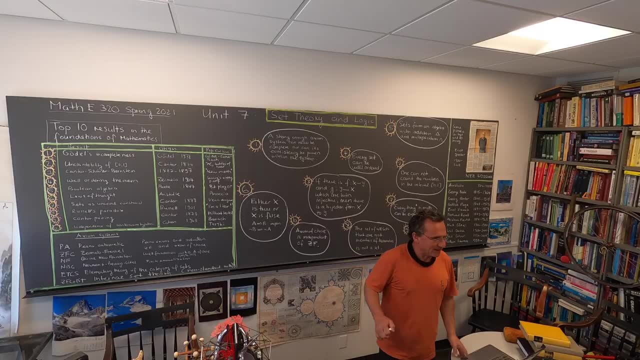 of the integers, so you can count them: 1,, 2,, 3,, 4,, 5.. And then there's the infinity of the interval, or the infinity of our space, And these are different infinities. So it's definitely fine to think about infinity And it's a very beautiful argument, this diagonal. 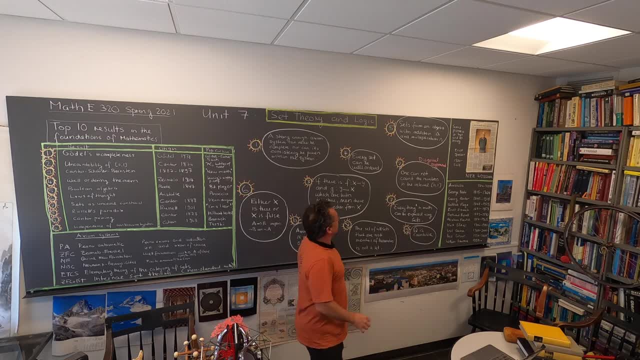 argument. Maybe I'll just make a few notes here. We can actually prove that for any set, 2 to the x has a larger cardinality than x itself. So all the power sets, the set of all subsets, has more sets in it than the set itself. 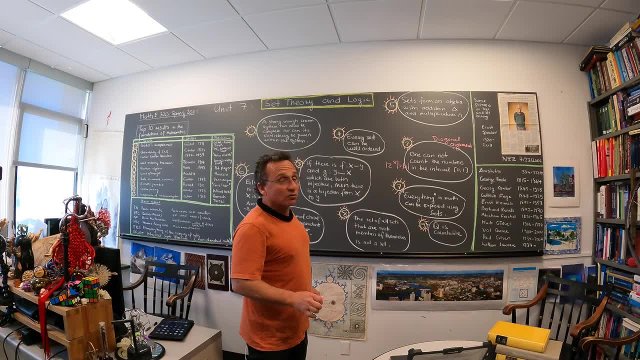 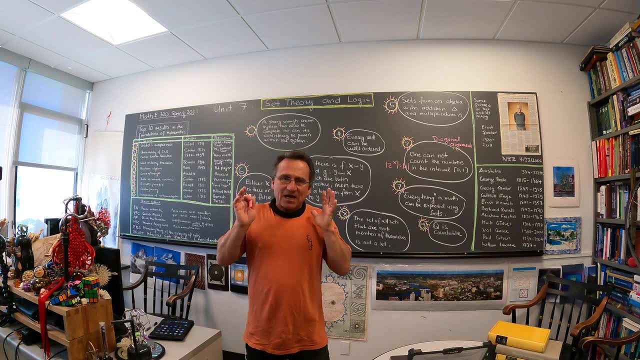 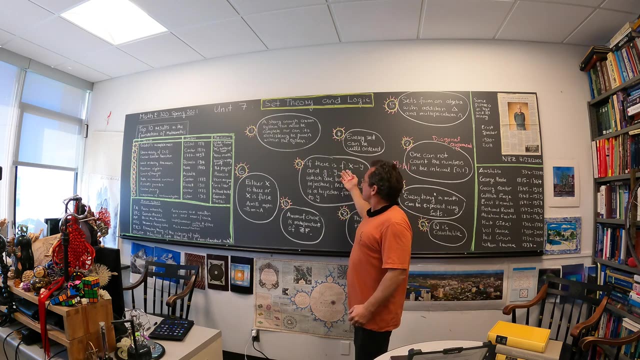 The third result is kind of something which Cantor assumed to be true but he only proved it later And it's now called the Cantor-Schroeder-Bernstein theorem. It's actually very exciting because the notion of cardinality, that's what Cantor's big idea was- See a set x has less cardinality. 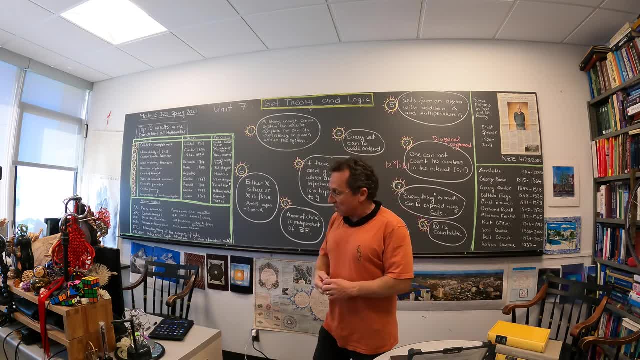 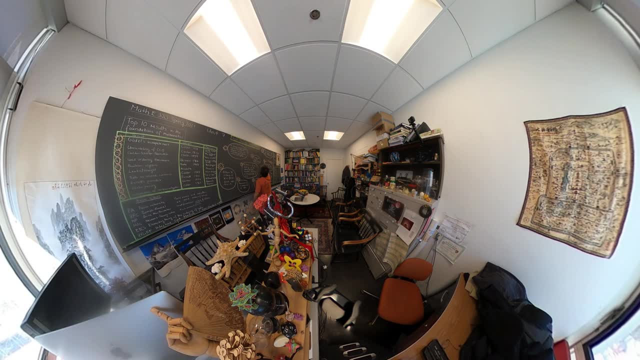 than a set y, And if there is an inductive function from x to y. so let me just say, maybe this is x and this is y. So if you can assign to every point x, you can assign a point here in y. 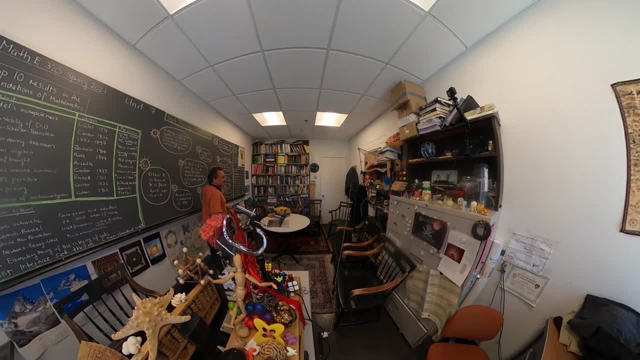 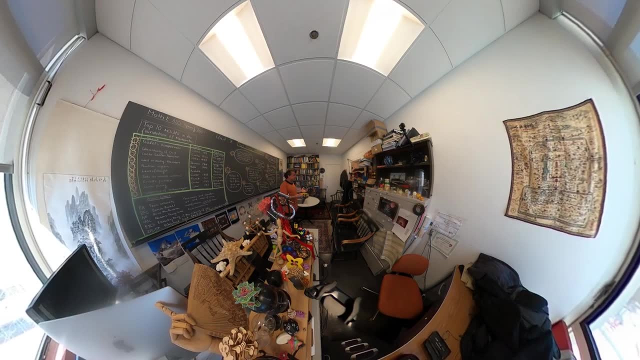 and you never have this possibility that you have a collision. You have not. this is not allowed. So this is called injective. Different points are mapped into different points here, And if you have that and you have also a reverse, if you have this, then you have a. 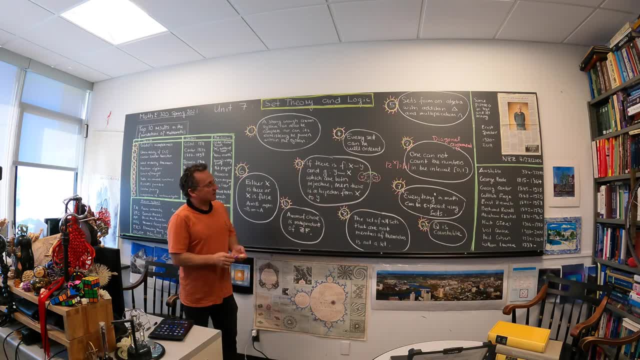 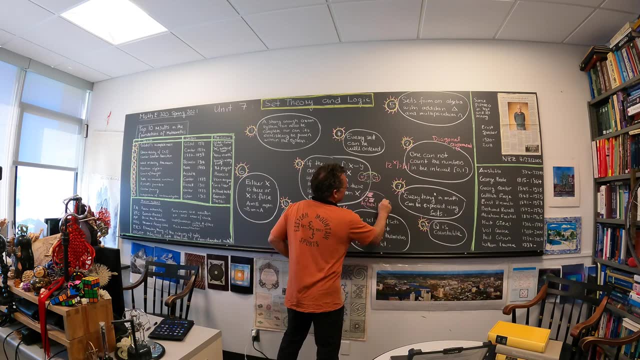 reverse, And then they have the same cardinality. See, so this is the Hilbert Hotel. So you think that the numbers 2,, 4, 6, the even numbers, these are the even numbers. you think that the even numbers there are less even numbers than an entire, than all the integers, because 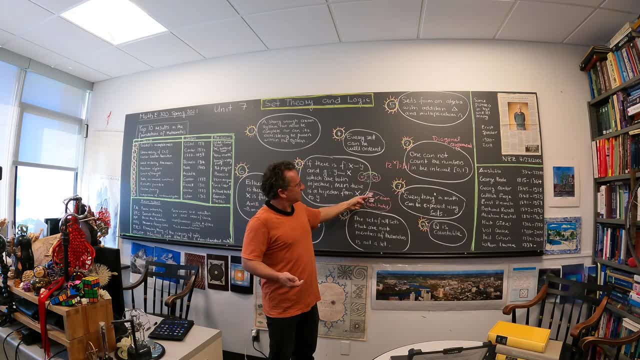 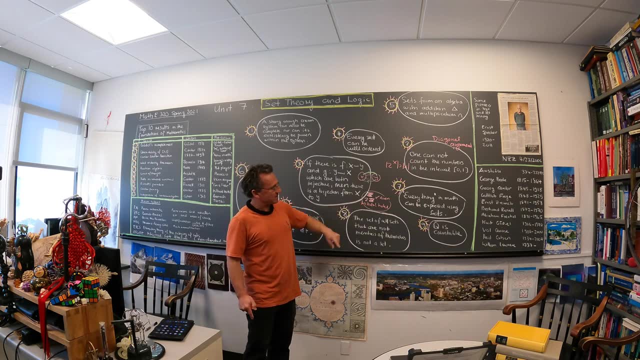 it's half of it, But you can find a bijection between these two things. You can map n to 2n in a one to one way, And so they have the same cardinality. So it looks less And then more surprising is that you also can count the rational numbers. 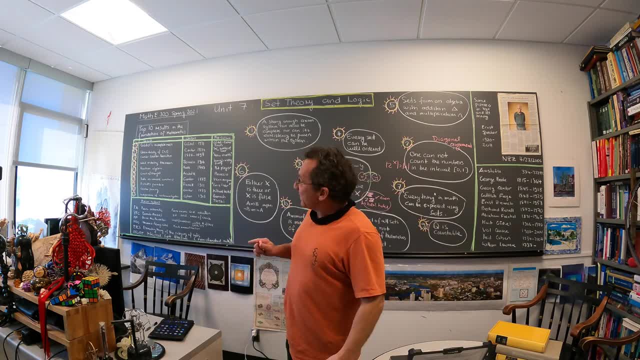 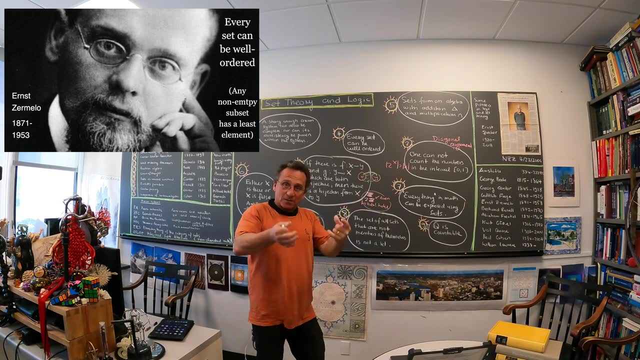 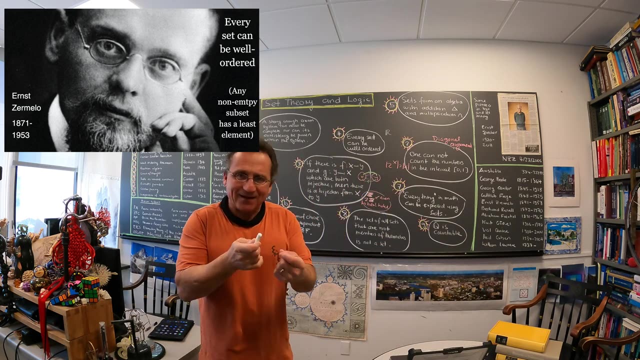 when you come to this, A very exciting theorem is the Zermelo theorem, which is a well-ordering theorem, which says that every set can be well-ordered so that every subset has a least element, But an explicit ordering, even for the reals, is not known in that way. This is equivalent to the axiom. 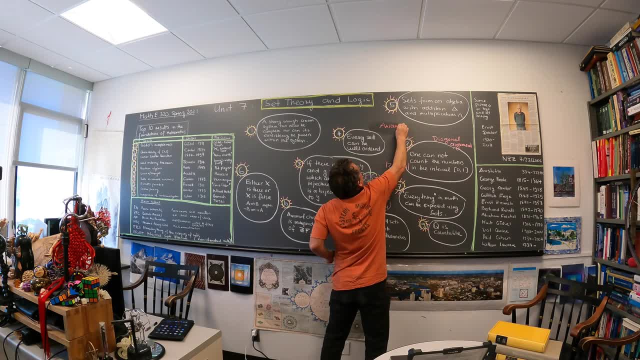 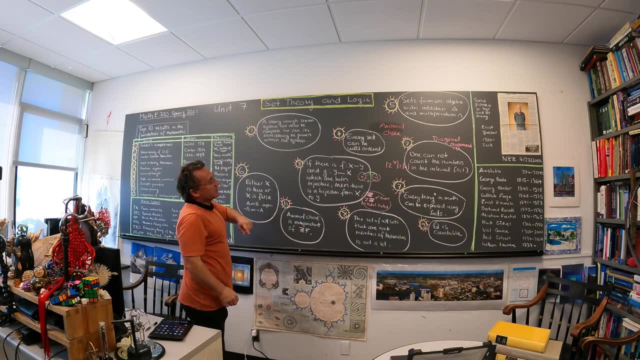 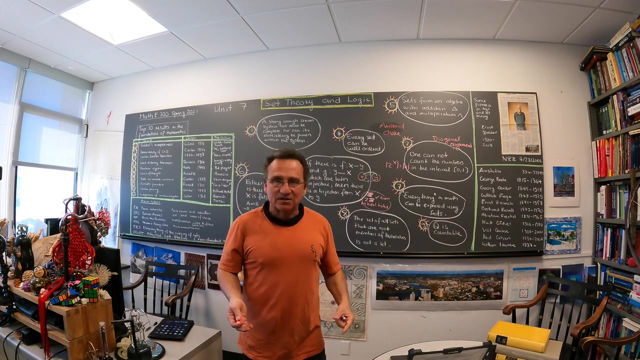 of choice, And the axiom of choice comes also back here in number 10.. So this axiom of choice is something we choose to actually accept And it has consequences, like the Banach-Tarski paradox. I will come to this just in a second. 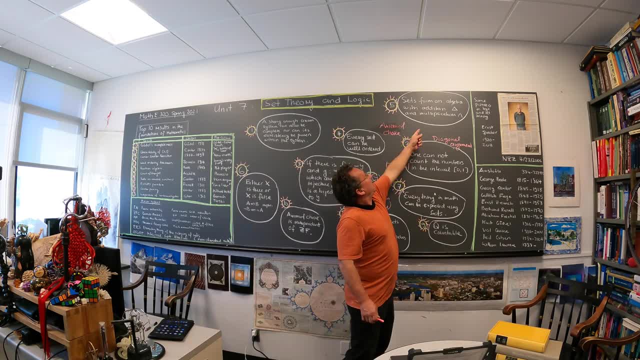 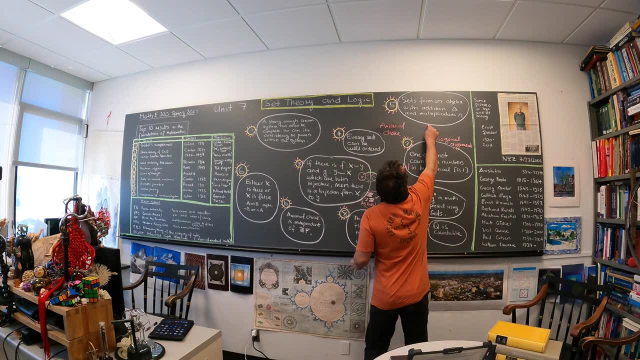 The next thing is very, very interesting. The next thing is very, very interesting. The next thing is very, very interesting. The next thing is very, very important. So we can form an addition of sets. So we can form an addition of sets. So this is the addition of these two sets here. So this is x plus. 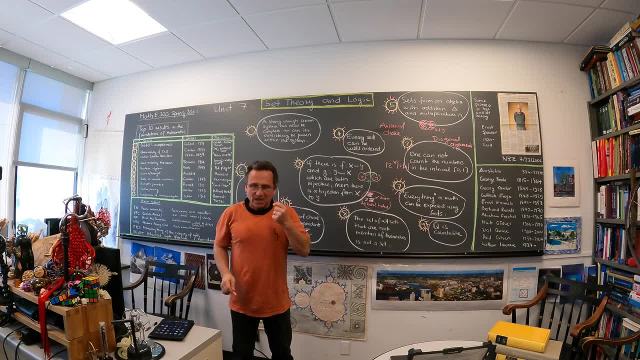 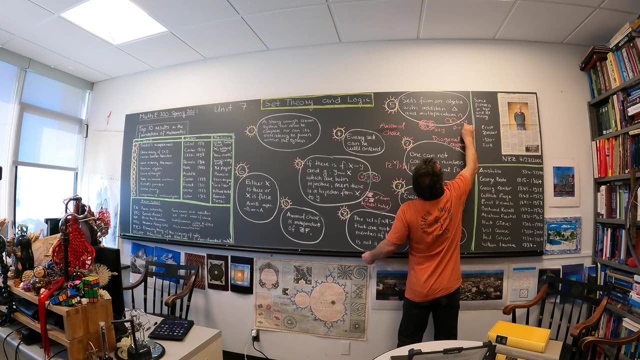 y, It's the symmetric difference, And the empty set is the zero element. And then there is also an intersect. The intersection is, when you take the intersection, this is the multiplication. So we have an additional multiplication, like with the numbers And what Boole realized. 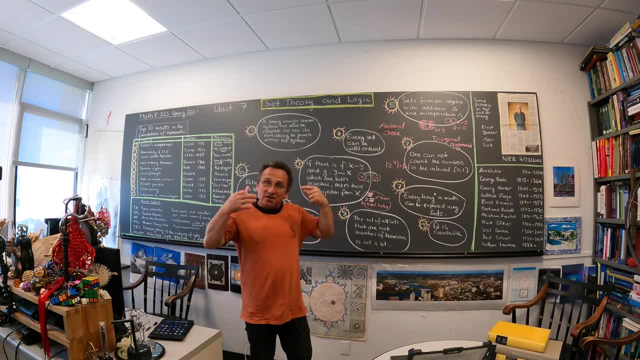 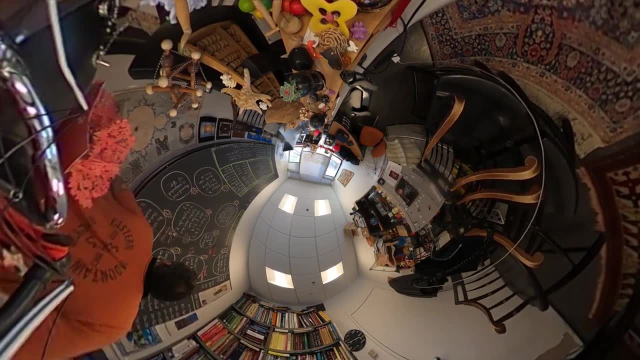 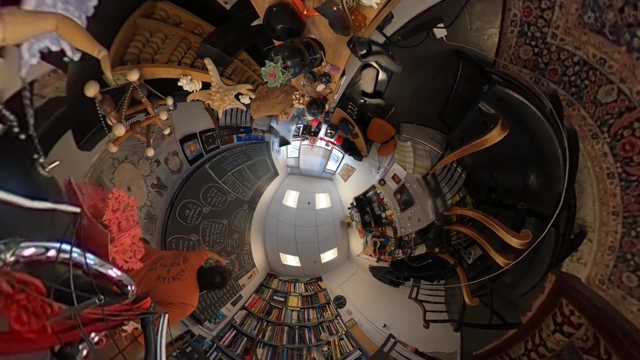 is. this is an algebra like the algebra of numbers And it has been reinvented again and again, like in computer science. Claude Shannon has actually his first paper- important paper as a student was about this Boolean algebra. It's very, very important in computer. 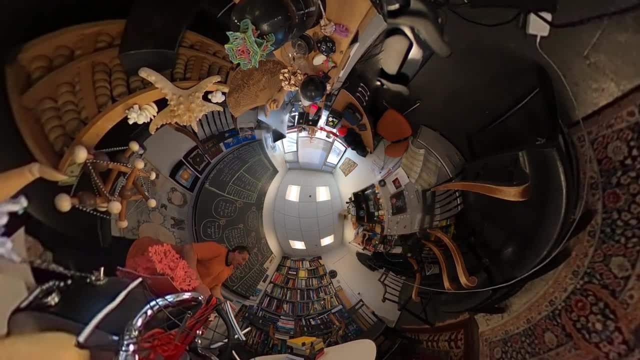 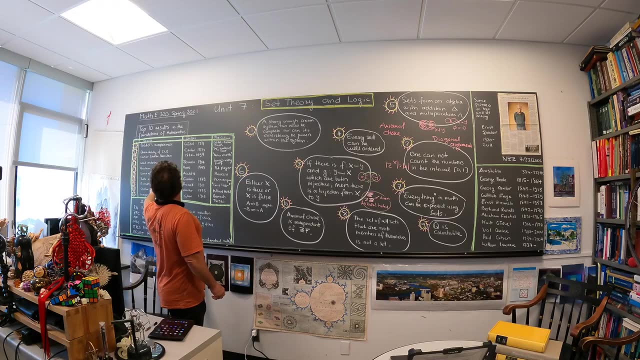 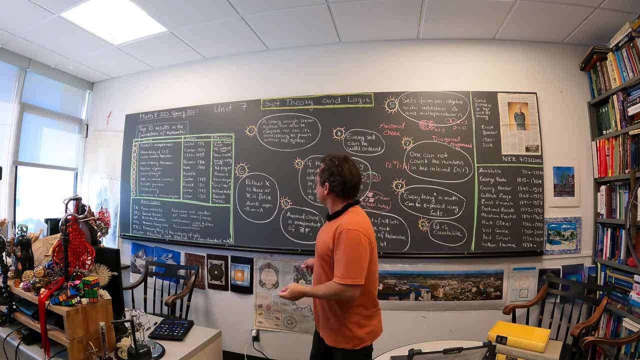 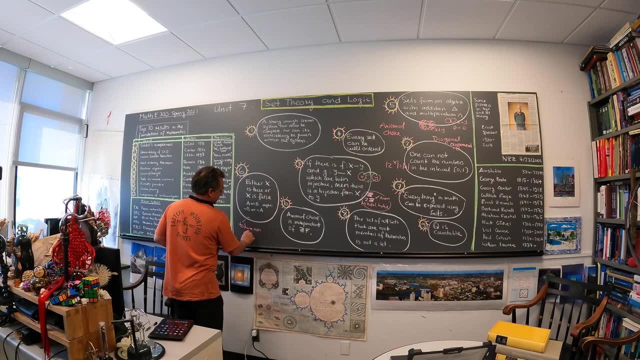 The next thing is the law of thought. So that's kind of the tertium non-dartor, for example, And it's very old Aristotle already. you know either something is true or something is false. right, But somehow there is a catch to it. We have things which we can choose. 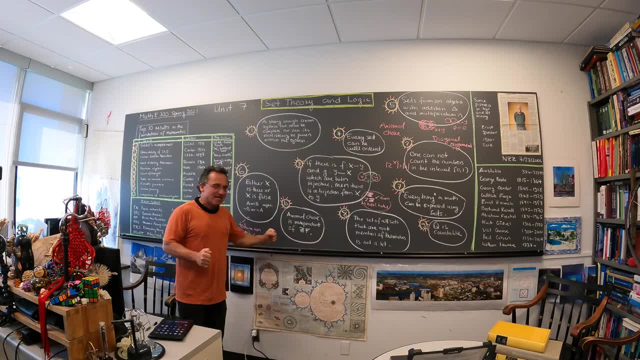 whether it's true or false. It's very exciting here We are really in a very, very exciting area of also philosophy- And so Aristotle was also a philosopher- And things like this: that if A implies B, then B need not. B implies not A, So this is not. So. you cannot reverse that Often things. 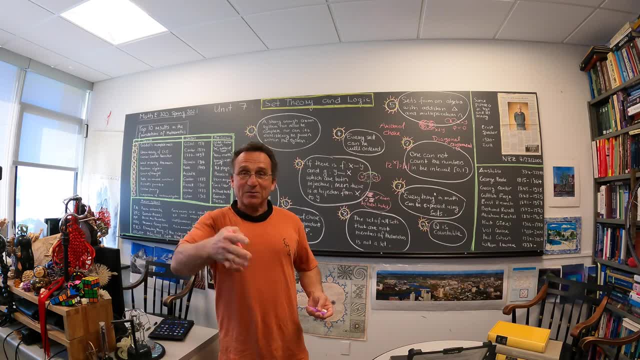 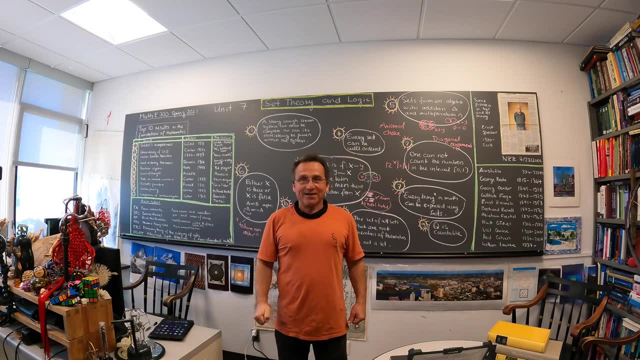 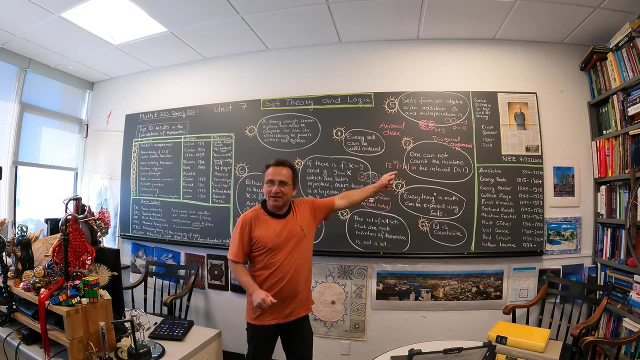 this is done wrong, also by politicians. If A implies B, it's not true that B implies A If it rains and the street is wet. But if the street is wet, it's not necessarily raining. right, You could have watered it with a hose. So that's an example of Specker. 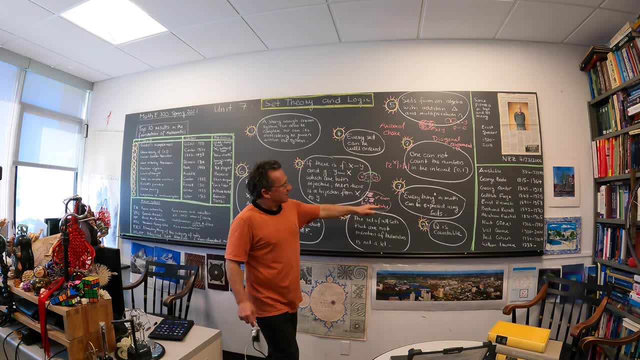 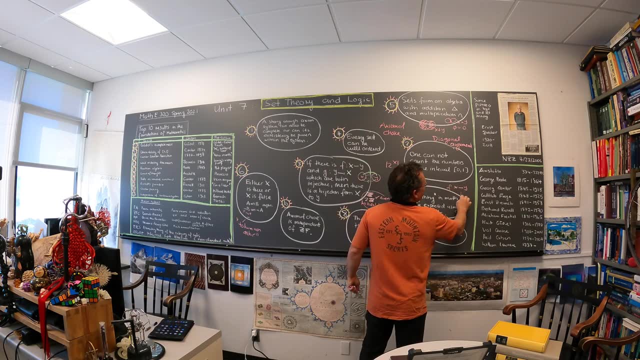 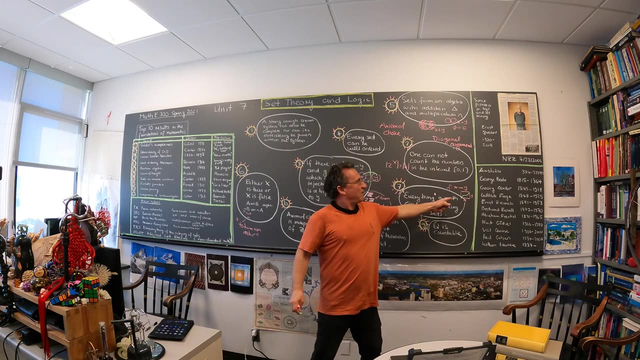 Now sets as a universal construct. that's very exciting also that we can, for example, say: if you have a function from x to y, we can represent it as a graph. This is x and y, And then we represent it as a graph. right, So we have represented this function again. 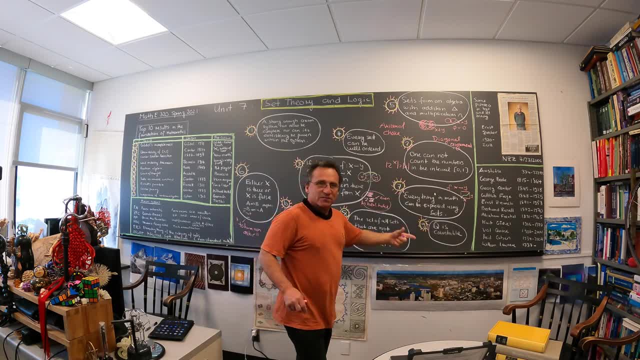 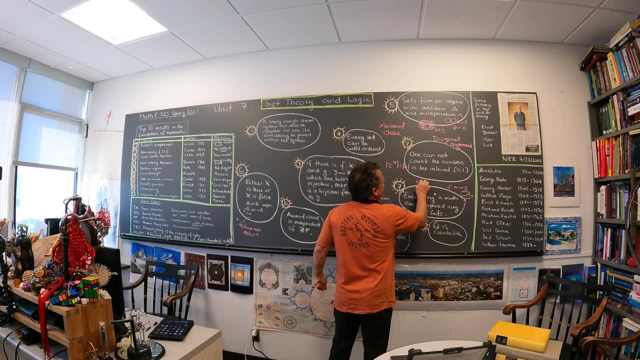 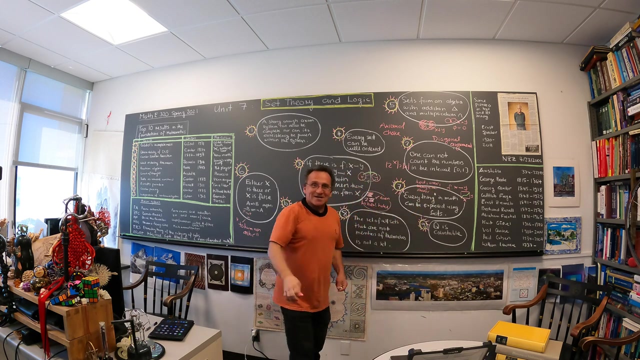 as a set. So we have topologies, we have sigma algebras, we have orderings, we have a lot of constructs, right, We have topological, we have order, we have measure, theoretical. So it is all these things which we have, all these shifts. whatever we define, we can do. 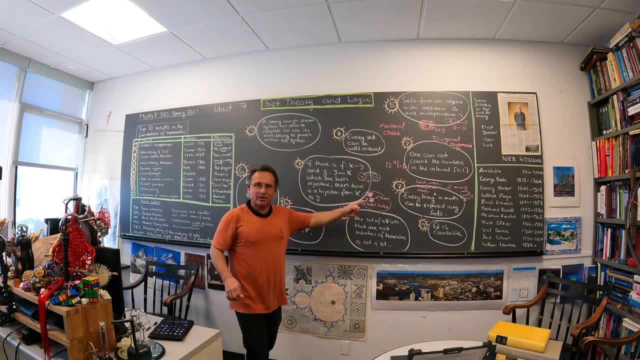 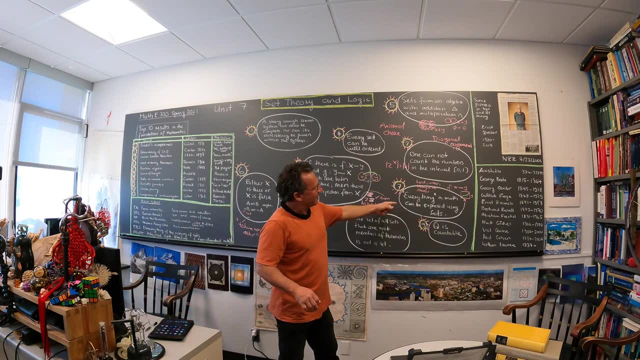 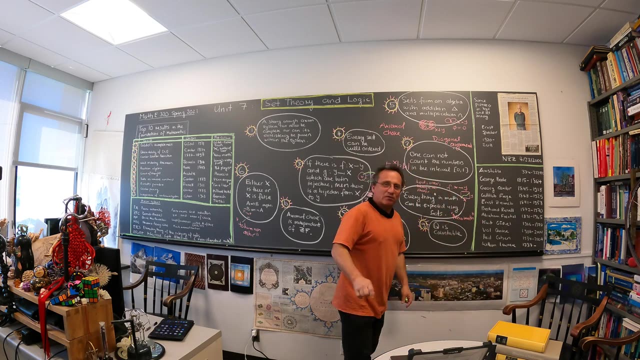 with the set theory, Similarly also with category theory, we come to this. So there are other alternative frameworks which also work. But it's kind of a from pop culture point of view. it's the new math thing that we have put the language of sets. 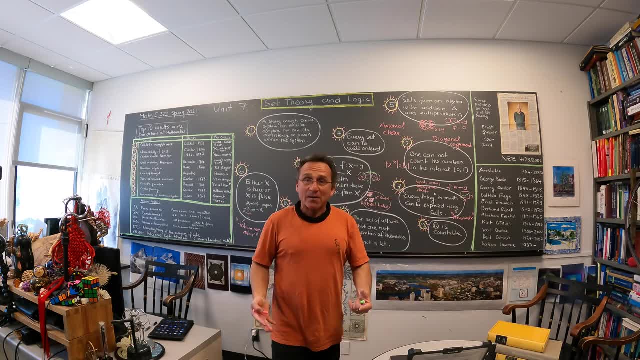 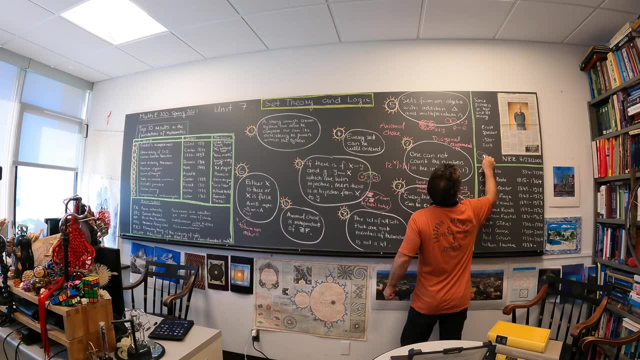 already very early in education. also, I was exposed to this in primary school, very early on and I found it very accessible. So sets, you see, if you take sets and so you make, you make. for example, the union of sets is Venn diagrams. 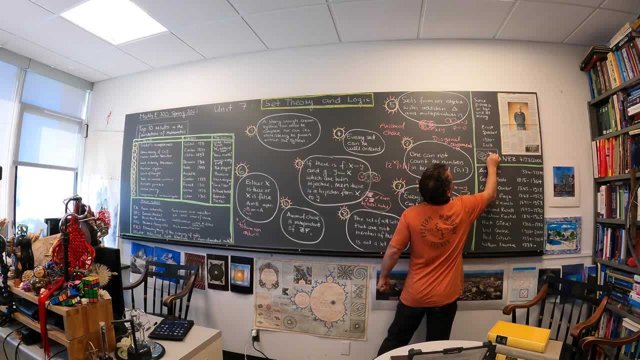 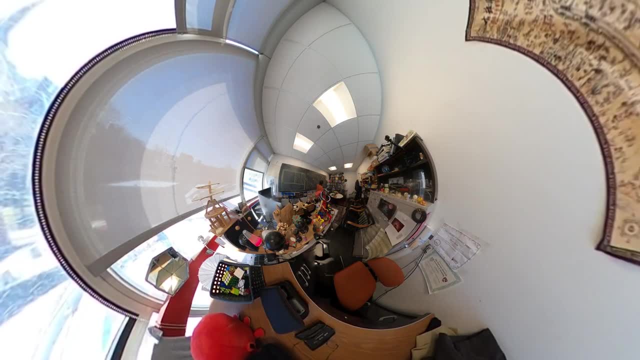 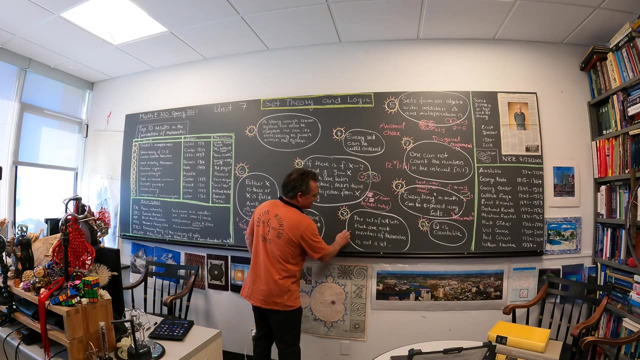 So this Venn diagram, this is something which is very accessible, even more than fractions, which comes usually later. Russell's paradox, So that's, that's very important, because this is a foundation of crisis- led to a crisis in mathematics. So can you really, if you have, if you have set. 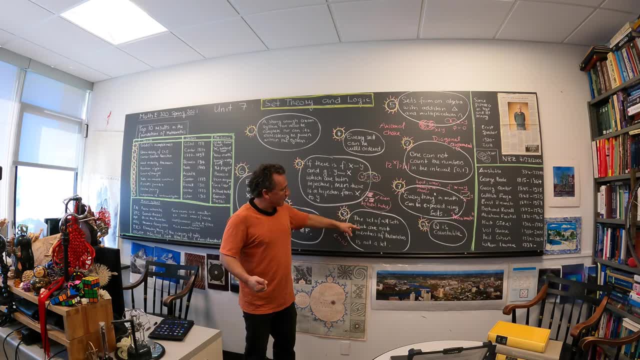 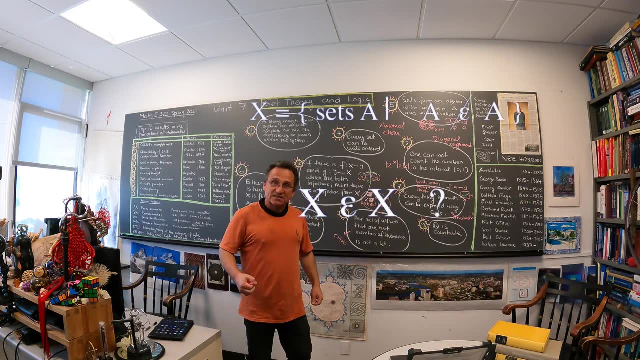 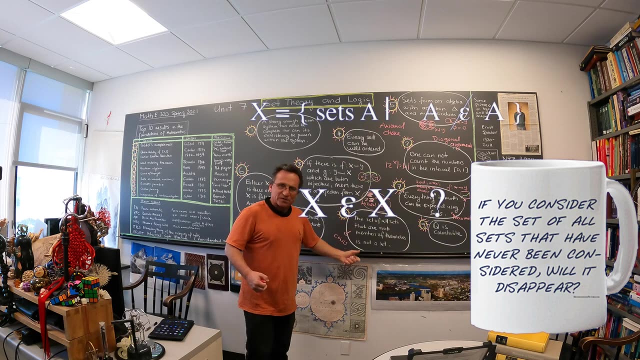 theory as a universal language. now you can define the set of all sets that are not themselves, not members of themselves, and you ask yourself: is this a set? So if this is a set, then it's not a set, and if it's not a set, then it's a set. So this is one of these paradoxes. 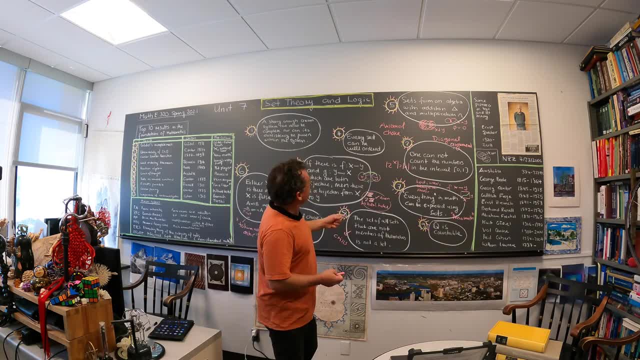 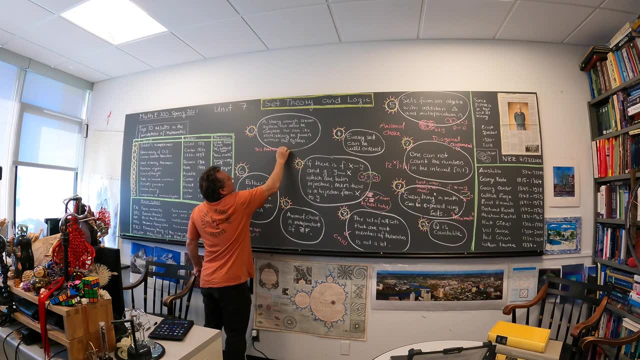 like the liar's paradox- I lie- or the paradox which actually is at the foundation of Gödel. this theorem cannot be proven, Which Gödel managed to formulate within the structure of mathematics. So you know, you formulate what is a theorem, what is a proof, and you make this: 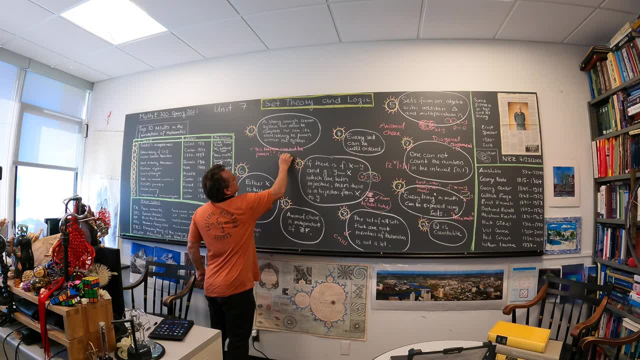 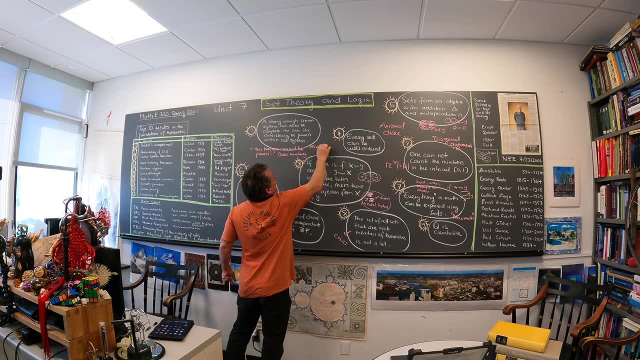 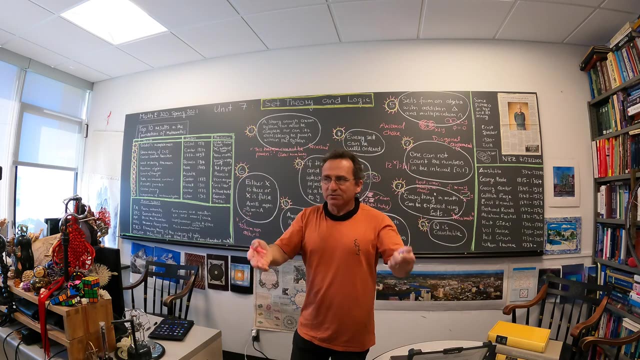 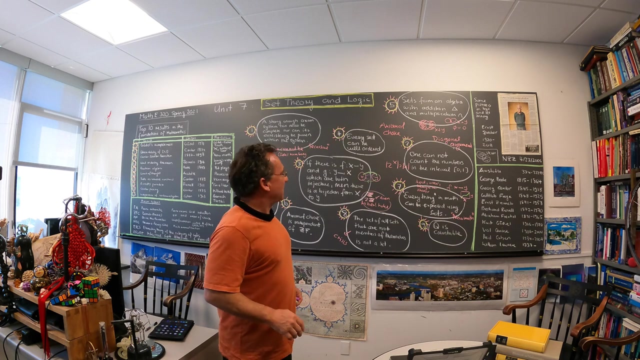 formalize this, and then you use Gödel numbering. So it's this recursive, this recursive idea, which is very well described in this Gödel-Escher-Bach, and it's in music, it's in art. Escher and Bach, both were very fond of this recursive theme. 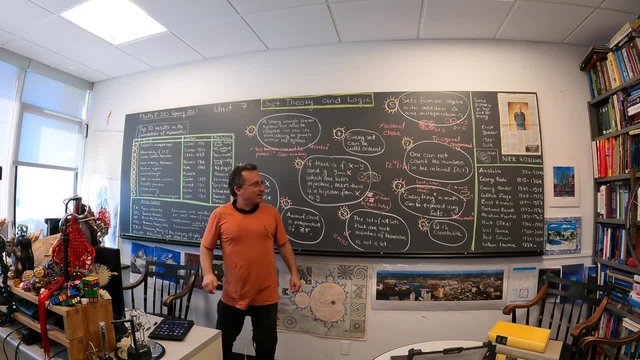 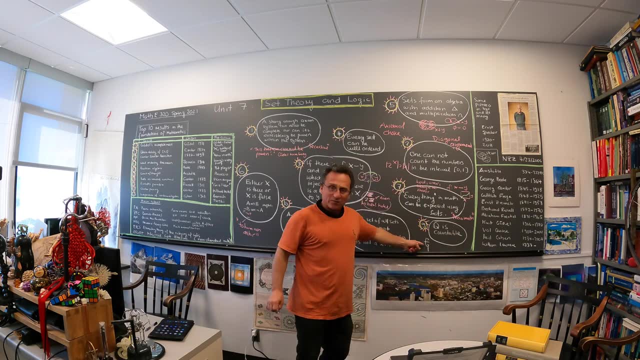 So that's the Russell paradox. Now, the contour pairing is an exciting thing that you would think that if you look at the fractions p over q, the p over q, the fractions p over q, they are actually dense in the interval. so every number can be approximated by fractions and it's a little bit. 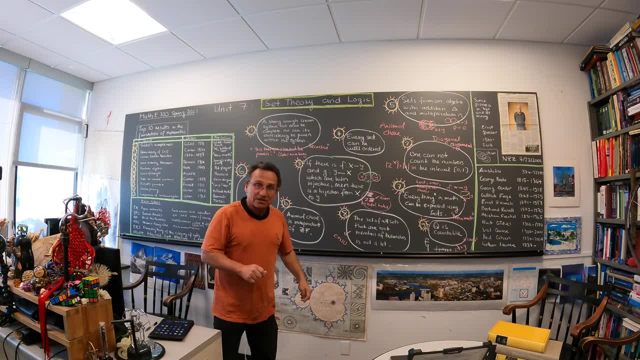 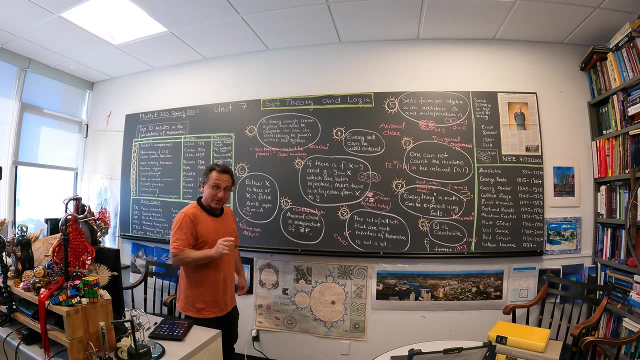 surprising, but a little bit, if you just I that you can count them. and finally, let's look at the Cohen theorem. So, axiom of choice, that's one of the things You can also say Continuum Hypothesist. So the Continuum Hypothesist is very exciting. the Continuum Hypothesist. 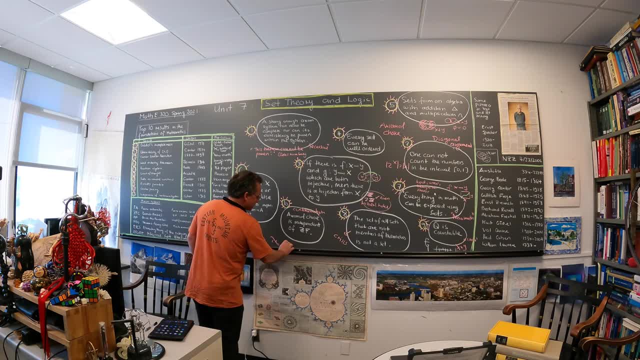 tells the aleph 0, between aleph 0 and aleph 1, which is 2 to the aleph 0.. so this cardinality, this is the cardinality of the integers and this is the cardinality of the reals. so whether there are is a cardinality between that, is there a cardinality between that? 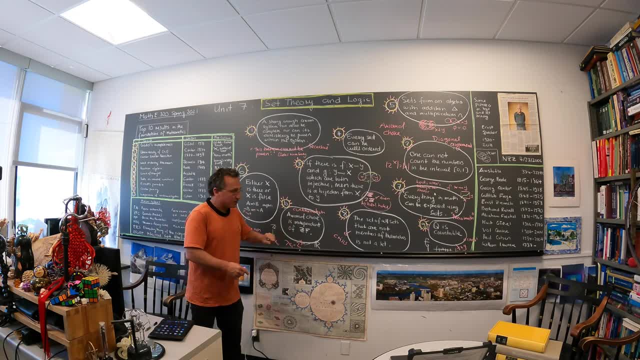 and Cohen showed in the in the 60s that it's it's, it's independent. so it's one of these examples which which Gödel kind of in his, in his incompleteness theorem, tells what you can. you can never really have a complete system. but it's surprising that also this continuum. 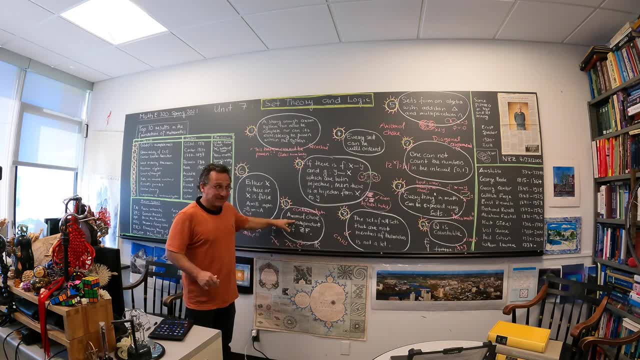 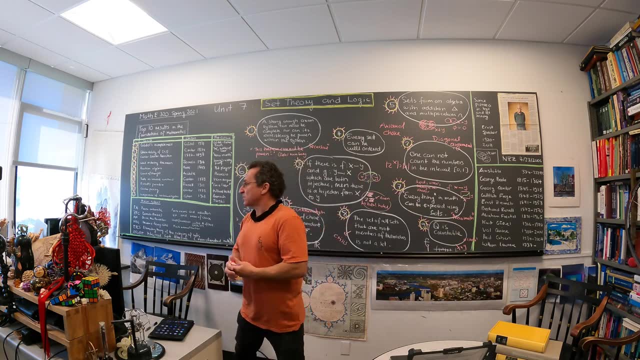 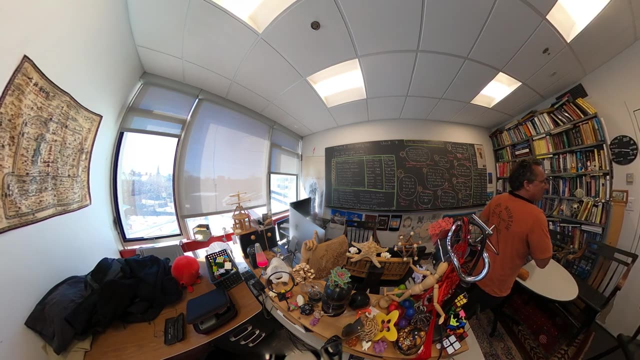 hypothesis is independent and the axiom of choice also. by the way, the axiom of choice is not very intuitive because what you can prove is: you can take. you can take a sphere like this and you can cut it into into five, five pieces. so maybe I take one piece, I take another piece. 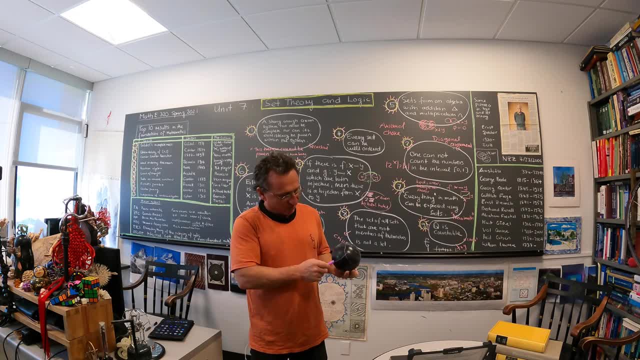 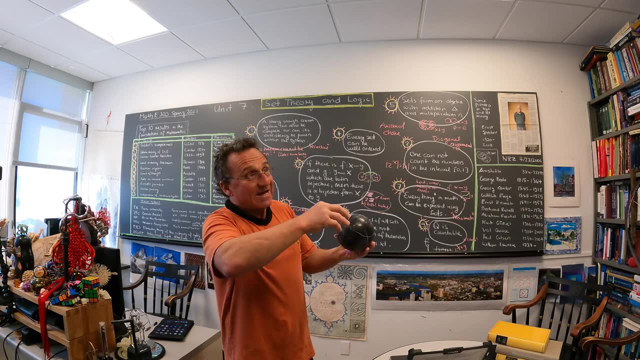 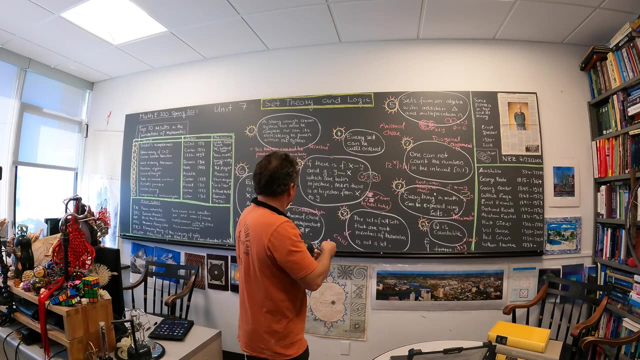 and I take a third piece and the fourth piece and the fifth piece, I can cut it into five pieces. this ball, I can cut into five pieces. I can cut it and and reassemble it, using translations and rotations only, and produce two spheres of the same size. so this is the, this is the Banach-Tarski. 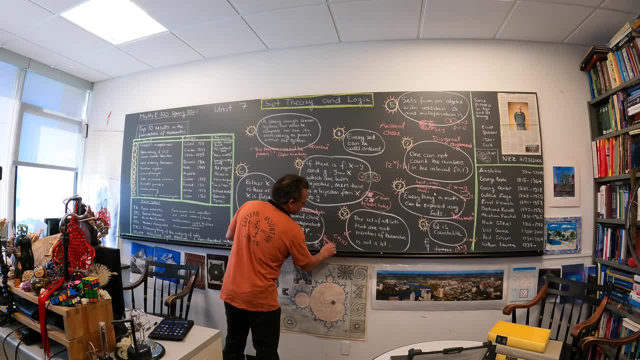 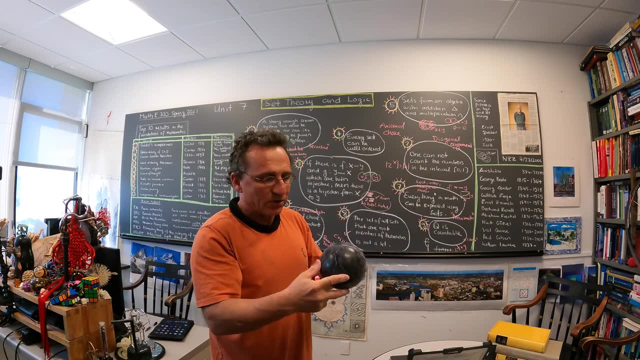 paradox, it's counterintuitive because we, we believe you know, if you have a, you cannot make out of one ball two balls, but you can make that. and it uses the axiom of choice and this shows also: there are sets which you cannot measure. you cannot assign a volume to this, to these sets. 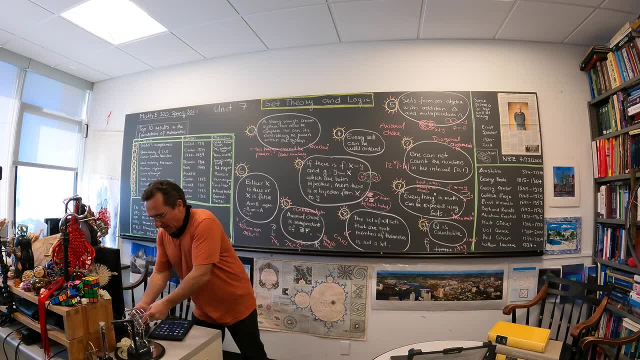 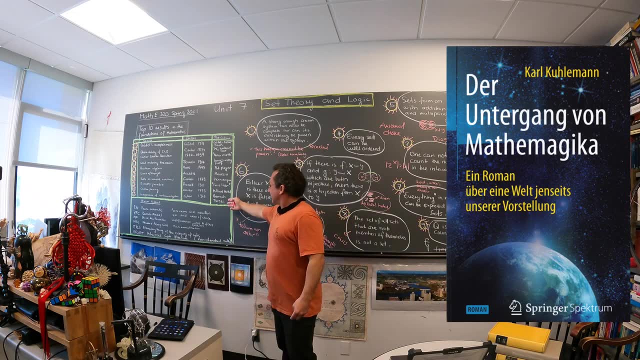 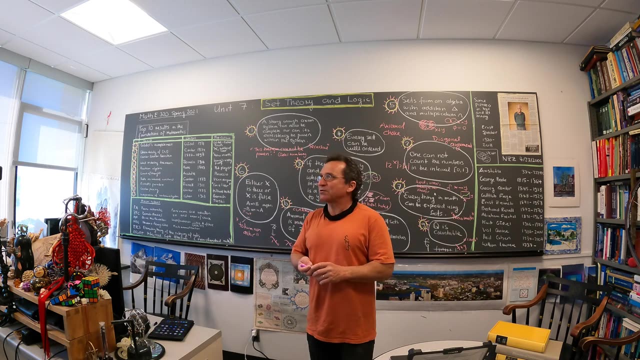 because the volume gets doubled. so that's very exciting and it's in in in the pop culture. there are books about that, novels about which have this Banach-Tarski paradox as a theme. cool, that's it. so I hope you enjoyed this video and I'll see you all in the next video today. 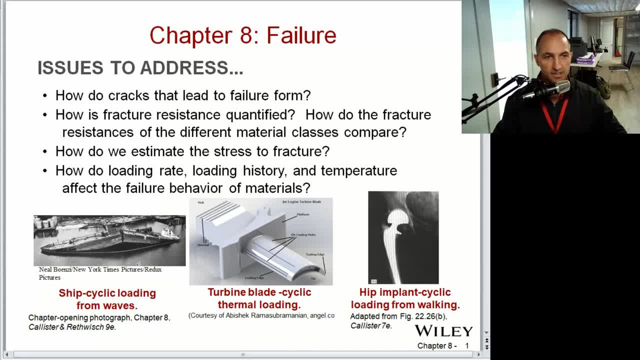 Hello everyone, This is Eric Payton Introduction to Materials Engineering, Chapter 8, Failure- Issues to address in this chapter. how do cracks that lead to failure form? How is fracture resistance quantified? How do the fracture resistances of different material classes compare? 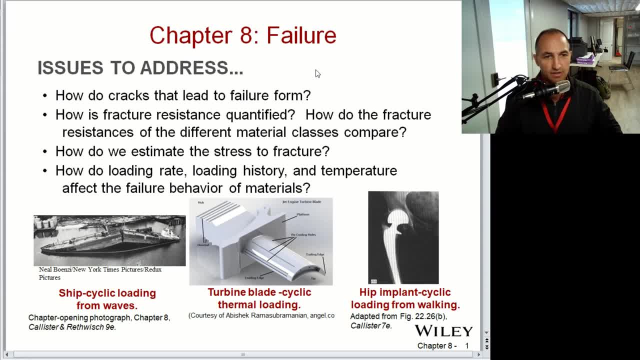 How do we estimate the stress to failure? How do loading rate, loading history and temperature affect failure behavior of materials? On the lower left, here we have a picture of a World War II ship And, as you can see, it is snapped completely in half. 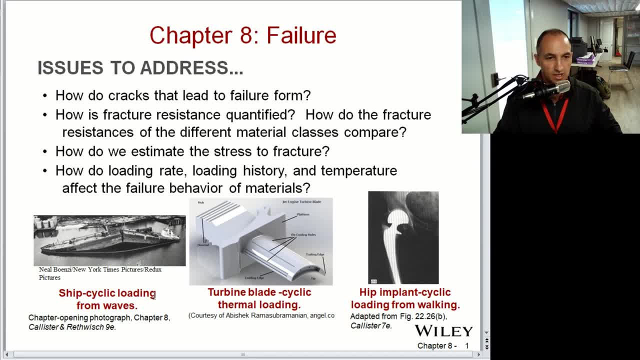 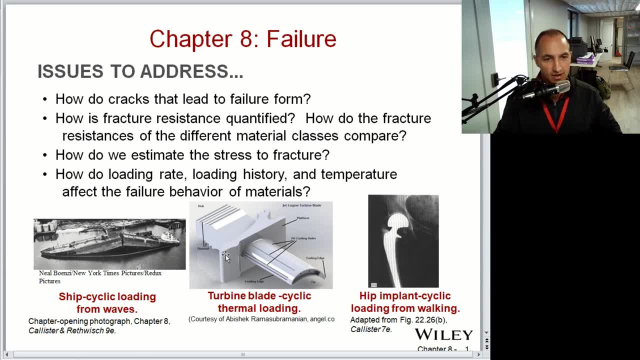 And this was due to ship cyclic loading from constant wave action. The middle picture here is an artist's 3D CAD drawing of a turbine blade, And this has thermal cyclic loading on this spin each time the engines start up and shut down. 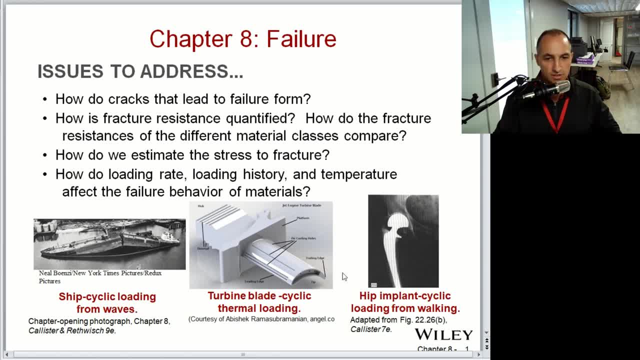 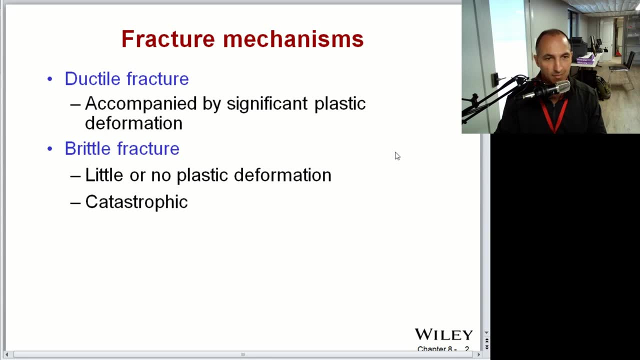 And on the right you have cyclic loading due to an artificial hip implant And this, as you've seen, is these two larger plates on the left. Here on the right, we have a feeler. This is 2,, 2,, 3,, 4,, 5.. And, as you can see, the entire site of the vehicle is stuck together. The entire frame of the vehicle is going to be attacked And, as you can see, the entire frame of the vehicle is going to be attacked. Now, if you are solving the case of a history class, you will have to re-examine and re-attach the plate.